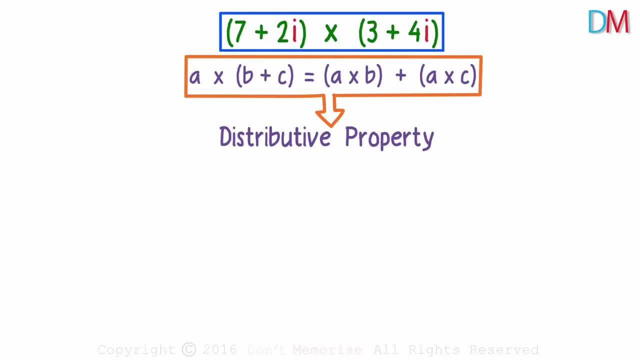 It's the distribution property, So this can be written as 7 plus 2i times 3 plus 7 plus 2i times 4i. Now focus on the first part: 7 plus 2i times 3.. It will be this number added thrice. 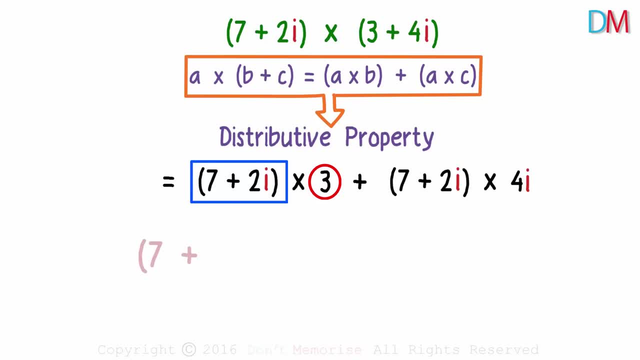 7 plus 2i can be added thrice to get 7 plus 7 plus 7 as real part and 2i plus 2i plus 2i as the imaginary part. This is 21 and this is 6i. 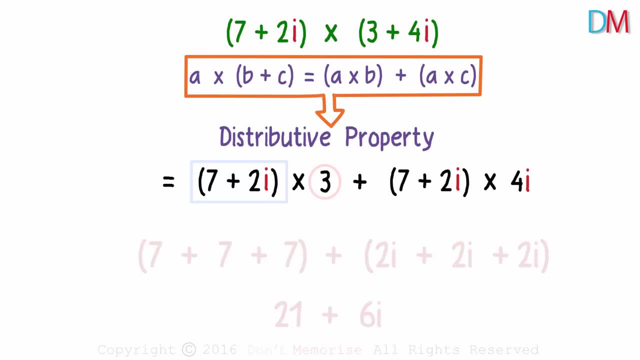 The result is 21 plus 6i. We actually use the distribution property here 7 times 3 plus 2i times 3.. 21 plus 6i. The second part is still pending. How do we account for multiplication of 7 plus 2i with 4i? 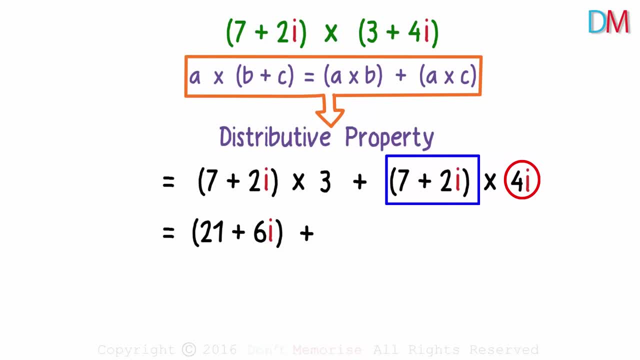 This added times 4i does not make sense, But we can still use the distribution property here. Multiplying 7 plus 2i with 4i, we get 28i plus 8 times i squared, which is nothing but 28i plus 8 multiplied by negative 1.. 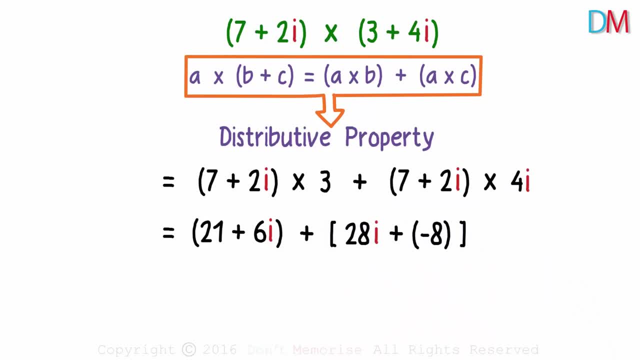 This is nothing but 28i plus negative 1.. This is nothing but 28i plus 8, multiplied by negative 1. This is nothing but 28i plus 8.. This is nothing but 28i plus 8.. This expression equals the product of these two complex numbers. 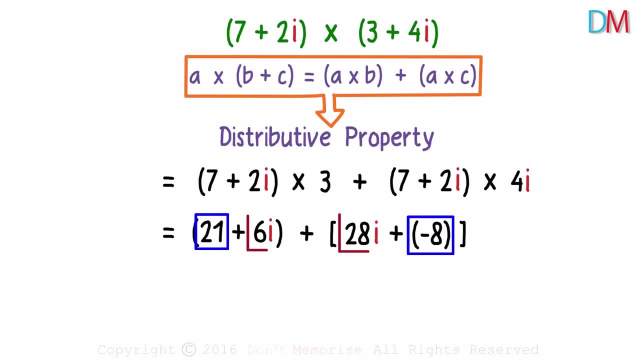 To get the final expression, let's add the real parts and the imaginary parts separately. We get the real part as 21 minus 8 and imaginary part as 6i plus 28i. Hence 7 plus 2i multiplied by 3 plus 4i gives us 13 plus 34i. 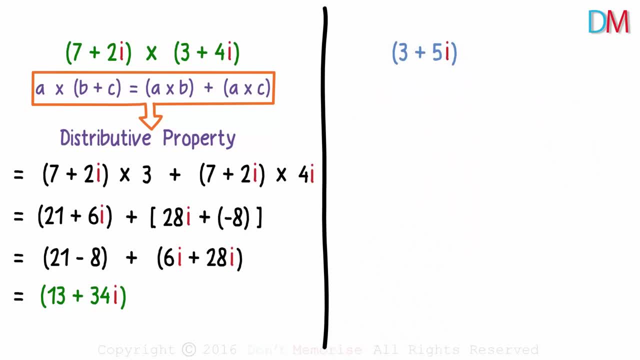 Let us pick up two more complex numbers- 3 plus 5i And negative 2 plus 4i- And work out their multiplication. Would you like to try it first? We can use the distribution property here to write this as 3 plus 5i times negative. 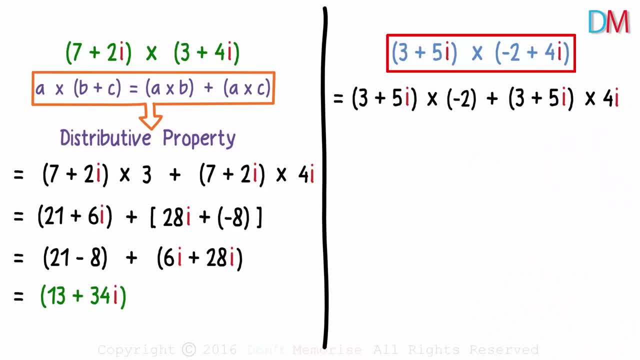 2 plus 3 plus 5i times 4i, 3 times negative 2 is negative 6.. And 5i times negative 2 is negative 10i. We get negative 6. And we get negative 6 minus 10i.